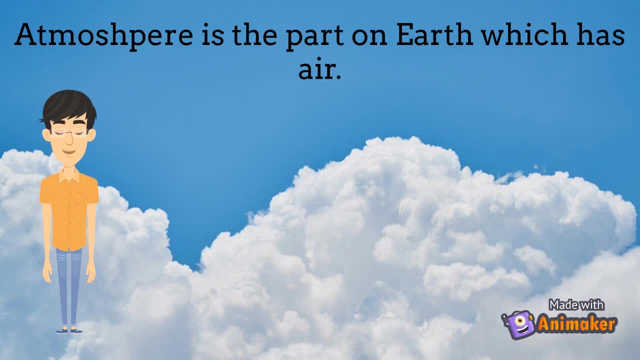 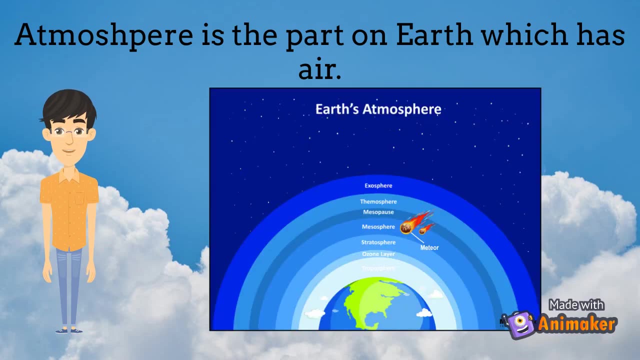 This includes winds, and it even includes the oxygen we breathe: carbon dioxide, hydrogen, nitrogen and others. Earth's atmosphere consists of seven layers, which are the exosphere, thalmosphere, mesopause, mesosphere, spectrosphere, ozone layer and peripersphere. 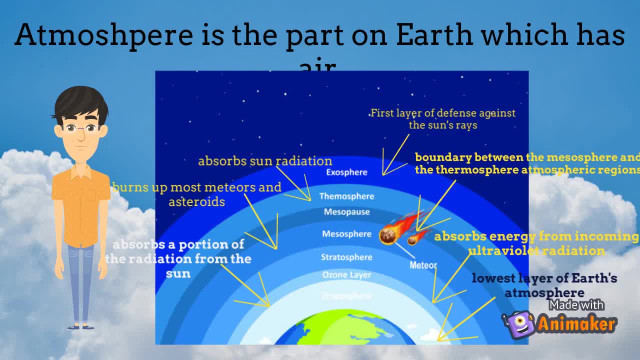 Now I'm going to tell you what each layer is about. The exosphere is the planet's first line of defense against the sun's rays, comet rays and asteroids. The thalmosphere is the fourth layer of Earth's atmosphere, which absorbs the sun's radiation, making it very hot. 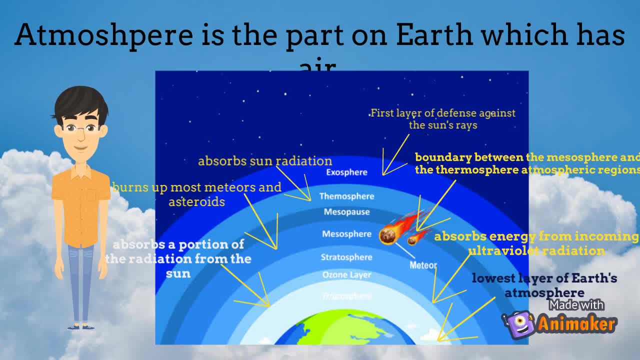 The mesopause is the point of minimum temperature at the boundary between the mesosphere and the thalmosphere atmospheric regions. The mesosphere burns up most meters and asteroids before they are able to reach the Earth's surface. The stratosphere absorbs energy from incoming ultraviolet radiation from the sun. 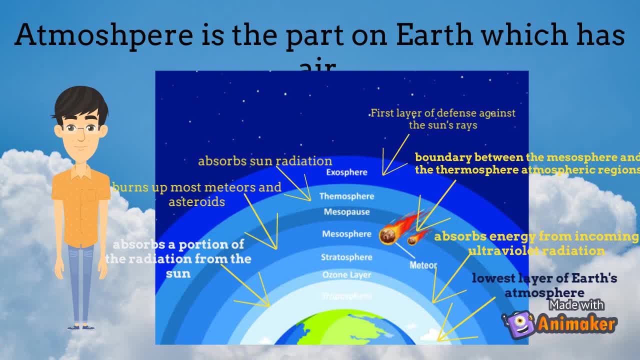 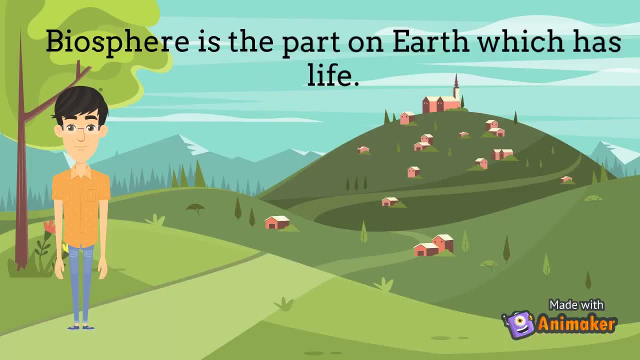 The ozone absorbs a portion of the radiation from the sun, preventing it from reaching Earth's surface. The troposphere is the lowest layer of Earth's atmosphere. Many types of clouds are formed here. Now let's move on to biosphere, which is the part of Earth which has life. 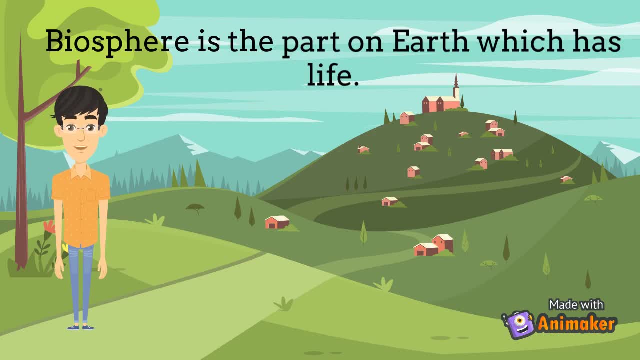 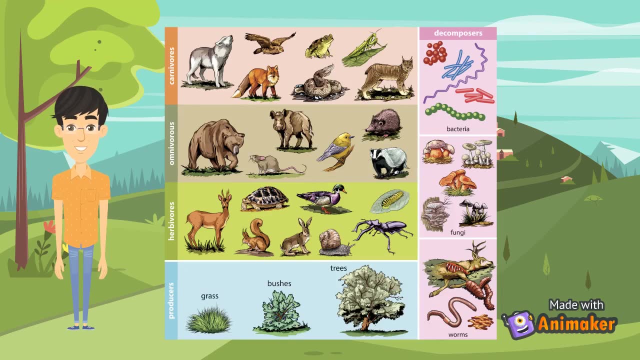 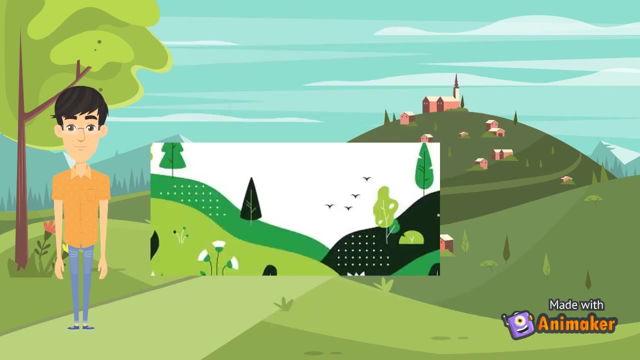 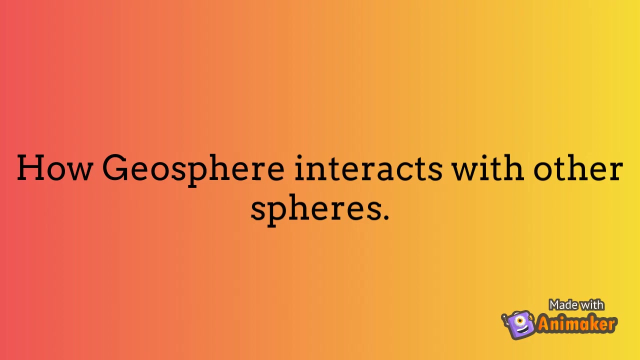 This includes humans, plants And animals. The place where an animal lives is called an ecosystem. The place where a plant lives is called a soil. Now I'm going to tell you how geosphere interacts with other spheres like biosphere, atmosphere and hydrosphere. 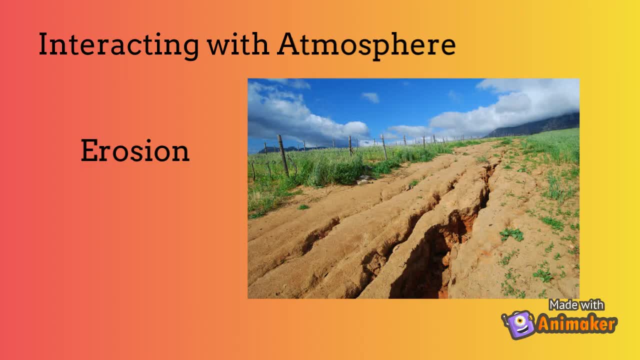 An example of a geosphere is the atmosphere. An example of a geosphere is the atmosphere. An example of how a geosphere interacts with the atmosphere is erosion. In erosion, materials are worn away and transported by natural forces such as wind or water. 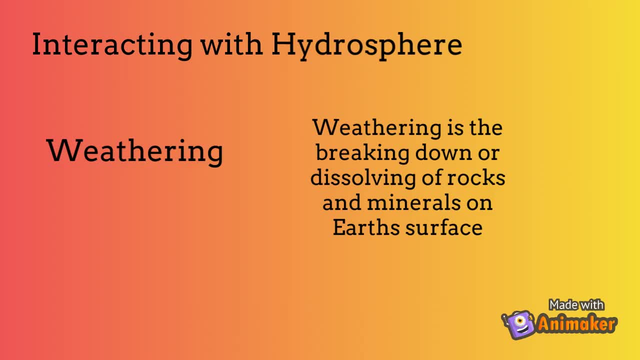 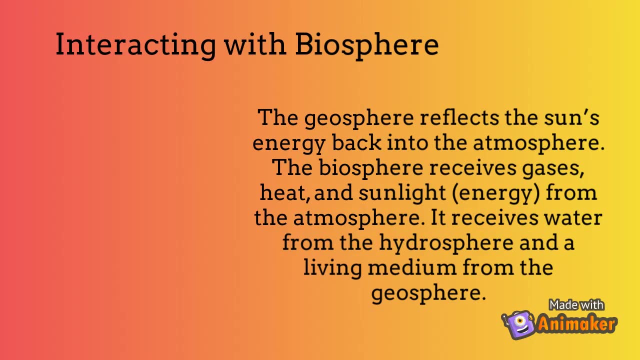 An example of how a geosphere interacts with a hydrosphere is weathering. Weathering is the breaking down or dissolving of rocks and minerals on Earth's surface. An example of how a geosphere interacts with a biosphere is that a geosphere reflects the sun's energy back into the atmosphere. 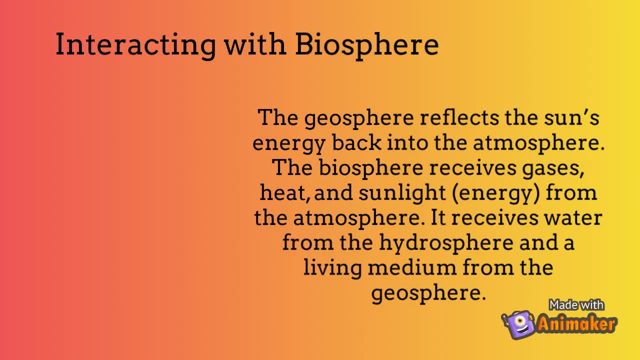 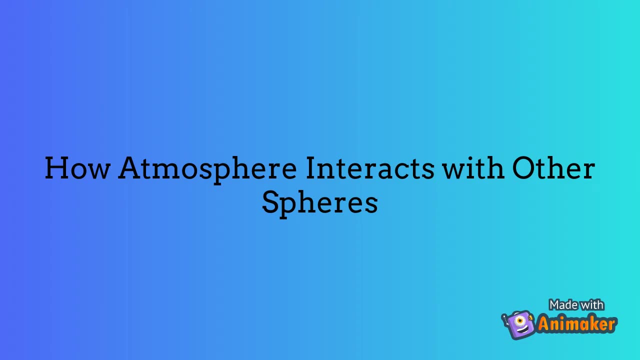 The biosphere receives gases, Heat and sunlight from the atmosphere. It receives water from the hydrosphere and the living medium from the geosphere. Now I'm going to tell you how atmosphere interacts with the other spheres, which are hydrosphere, geosphere and biosphere. 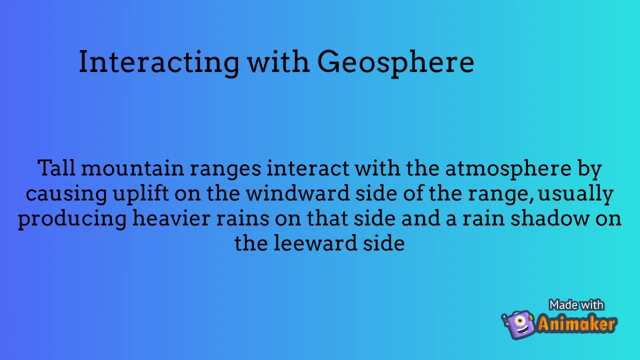 An example of how atmosphere interacts with the geosphere is that tall mountain ranges interact with the atmosphere by causing uplift on the windward side of the atmosphere, The wind usually producing heavy rains on that side, and the rain shadow on the leeward side, where it is so dry and gets less rain. 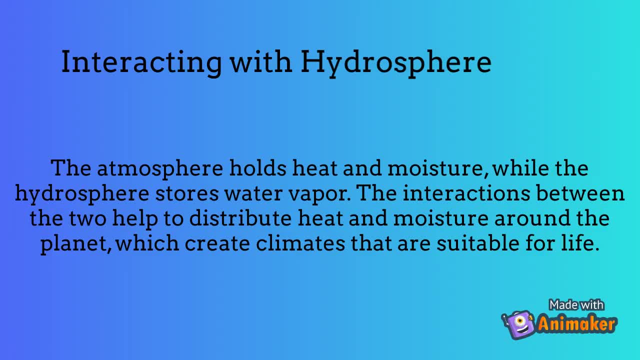 An example of how atmosphere interacts with the hydrosphere is that the atmosphere holds heat and moisture, while the hydrosphere stores water vapor. The interactions between the two have to distribute heat and moisture around the planet, which creates climates that are suitable for life. 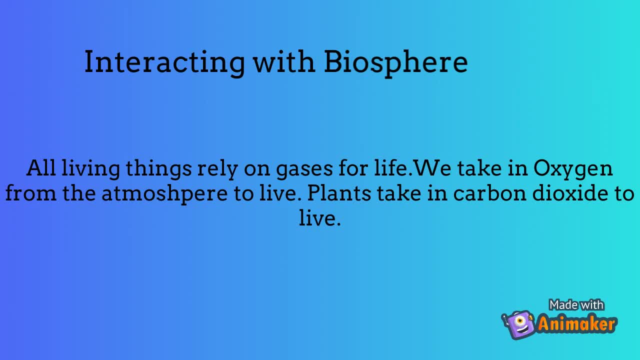 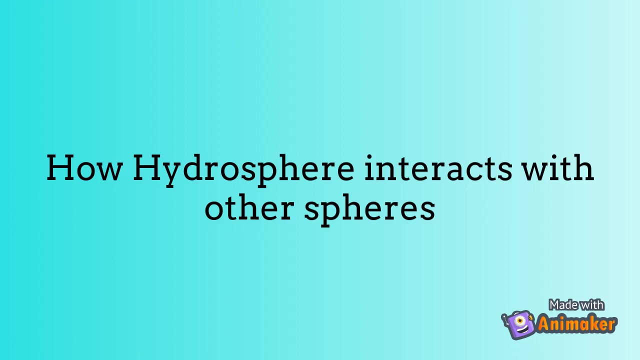 An example of how atmosphere interacts with biosphere is that we rely on gases for life. We take in oxygen for life and plants take in carbon dioxide for their life. Now I'm going to tell you how hydrosphere interacts with biosphere, geosphere and atmosphere. 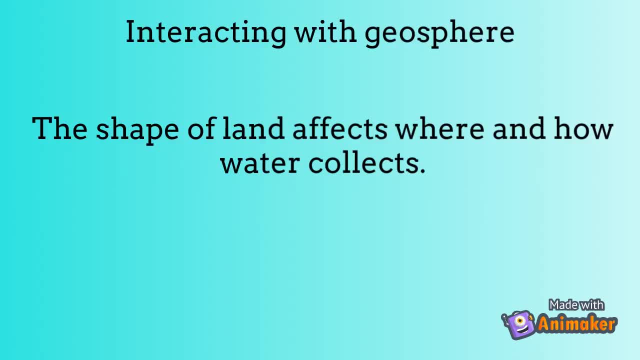 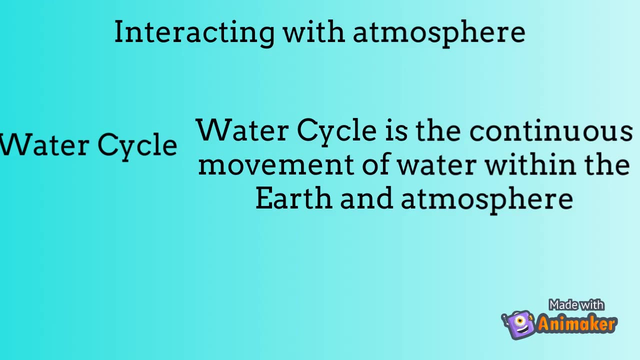 An example of how hydrosphere interacts with the geosphere is that the shape of land affects weight and how the water collects. An example of how hydrosphere interacts with the atmosphere is the water cycle. The water cycle is the continuous movement of water within the earth in the atmosphere. 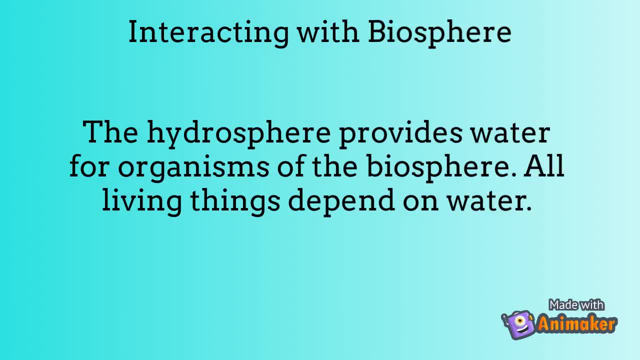 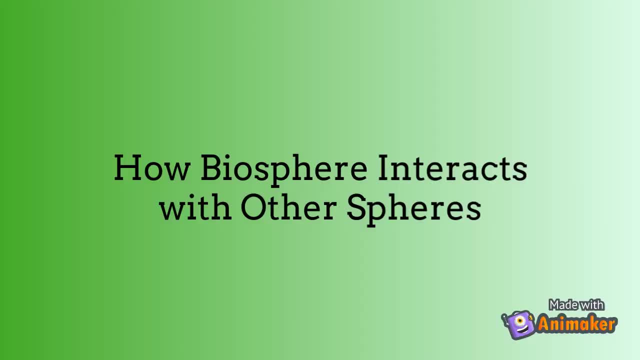 An example of how hydrosphere interacts with the biosphere is that the hydrosphere provides a variety of organisms in the biosphere. living things depend on water. Now I am going to tell you how biosphere interacts with geospheres. 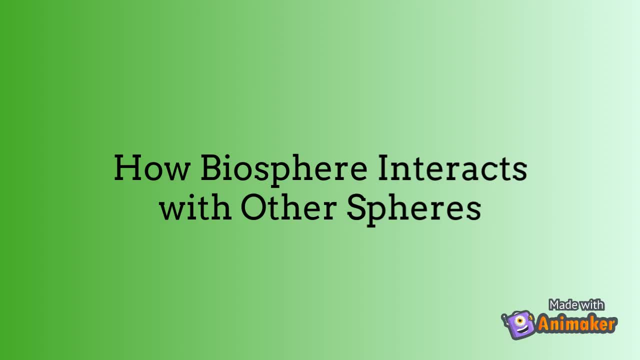 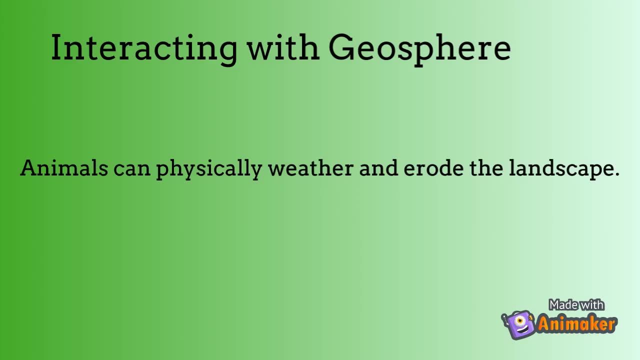 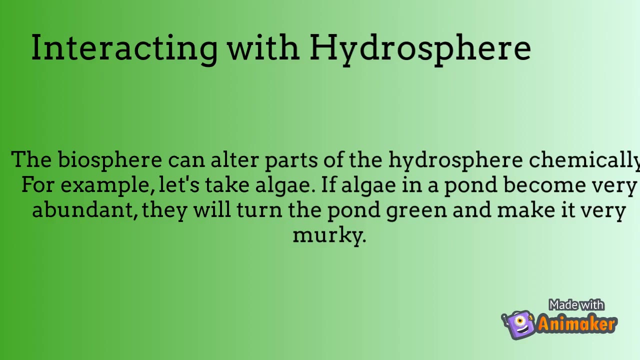 which are geosphere, hydrosphere and atmosphere. Now I am going to tell you how the biosphere interacts with the geosphere. Animals can physically rattle in the outer landscape, such as volcanic islands. Now I am going to tell you how the biosphere interacts with the hypersphere.